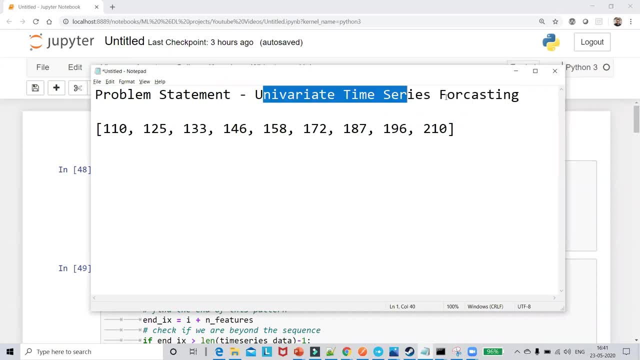 So the problem statement over here is that we are going to do a univariate time series forecasting. Okay, now suppose I have a company And I'm just taking as an example. And suppose there is a company And on the first day it has made this much sales: Okay, in the second day it has made. 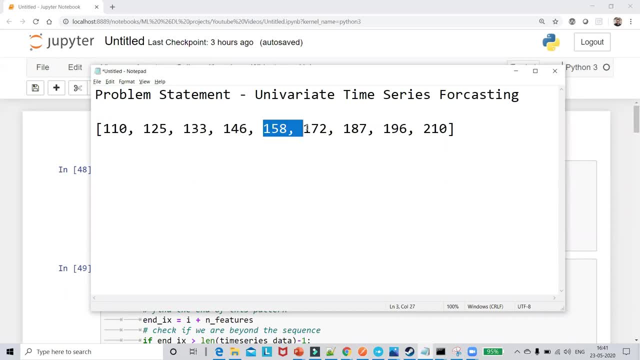 this much. sales In the third day this much. fourth day this much. fifth day this much. sixth day this much. Seventh day this much. eighth day this much. ninth day, this much. And you may be thinking: 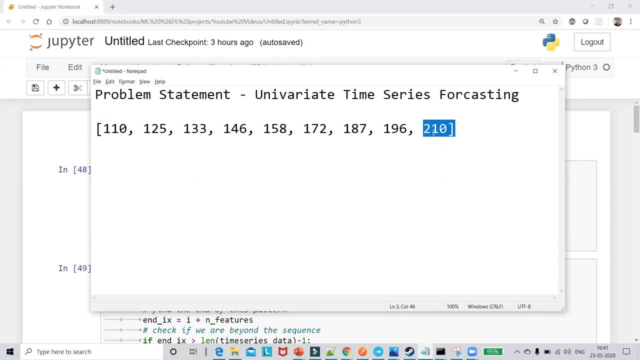 okay, Krish, why it is not reducing, Why it is always going into the in the positive direction may also have negative directions, right. It may also have some less number of values, right? So you may be thinking, Krish, why you're just taking these values? because this just seems to. 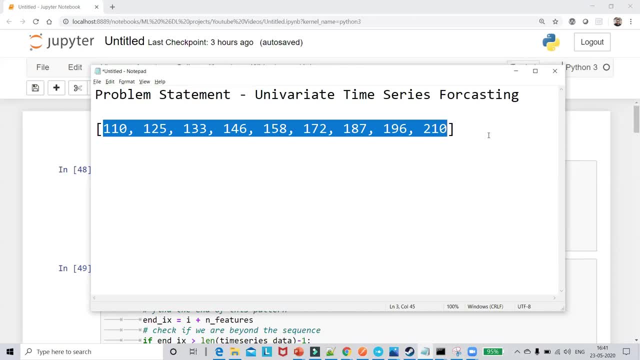 be increasing as we go ahead. So, but just by common sense, we can actually see that, yes, in the future also it will increase. It's okay, guys, you just take your own example, try to reduce this particular value And also see it's. it's just randomly, I've just selected. 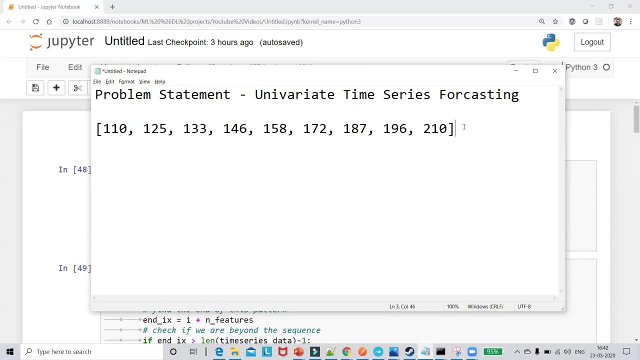 it. it is up to you, wish that, how you want to select this particular value. Now my problem statement is that considering the previous three days say okay, or considering the previous four days, or three days- let me just take three days- sales. I need to predict the next day, Okay. So 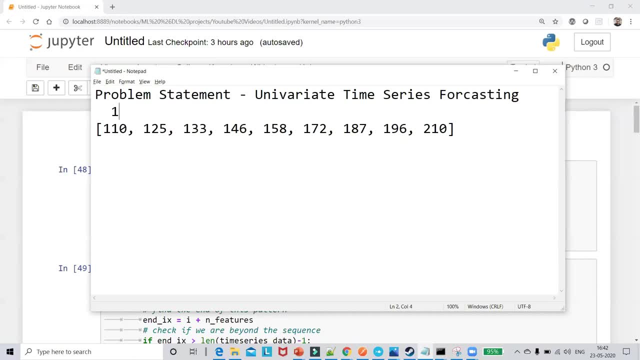 if I consider: over here, guys, I'll just write it down: This is my first day, This is my first day. Okay, oh, just a second. Okay, This is my first day. This is my second day. This is my third day. This is my fourth day. This is my fifth day. This is my sixth day, seven days. 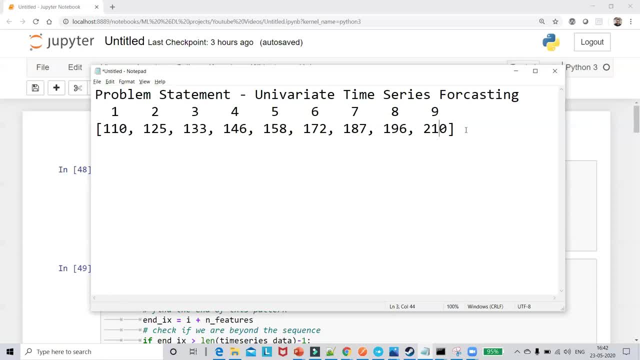 eight days and nine days. So what I have to do is that I have to do the prediction for my end day right, Considering the previous three values. okay, Considering the previous three values. Similarly, once I get my 10 day output, I similarly have to do for my 11 day, and here now I have to suppose my 10 day. 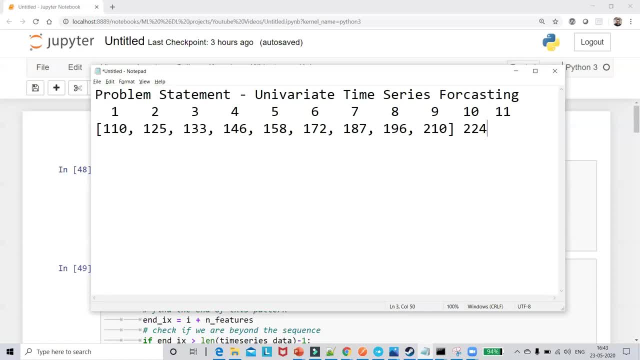 output. I've got somewhere around like 224. suppose I'll just take an example now for the 11 day. what I have to do is that I have to again take the previous three values and try to compute it. so, similarly, we will be doing continuously like this for the next 10 days, you know. so something like 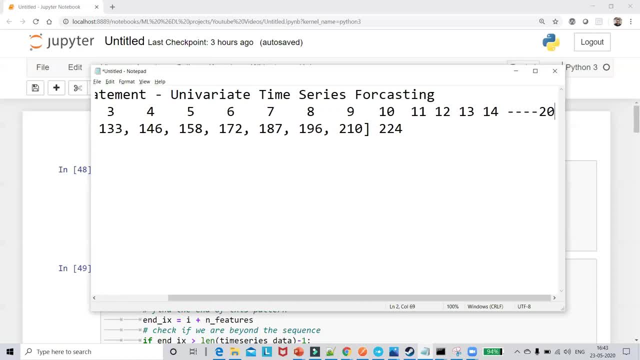 this up till the next 10 days, that is, up to the 28th day. so this is what is my problem statement now. first step that I really want to discuss about over here is basically the data preprocessing. okay, how we have to keep our independent and dependent feature, as I told you guys. 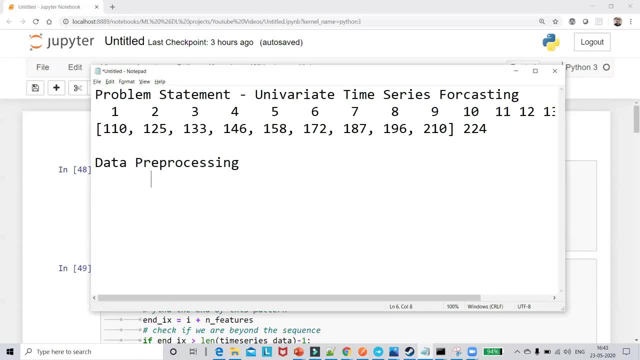 if I just consider, this is my x-axis. okay, now, if I'm saying that, my previous timestamp, I'm just going to consider three timestamps. so this will be my t1 type 3, 3 time. this will be my t2 time stamp. this will be my t3 time stamp. now i also have to create my 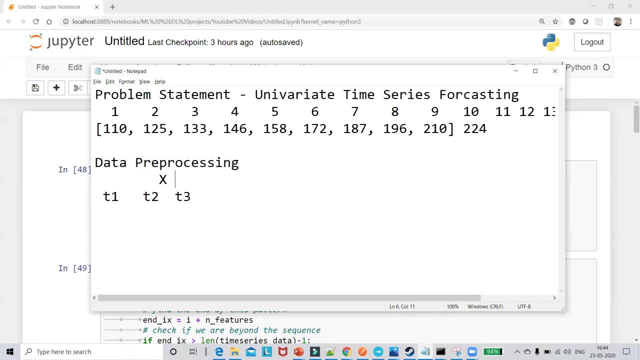 independent. so x is my independent features and here you have y is my dependent feature. so i also have to create my y value over here, which is my output. now how i will be actually creating it now, understand, guys, suppose? uh, this is my data set initially. i have first 10 days. 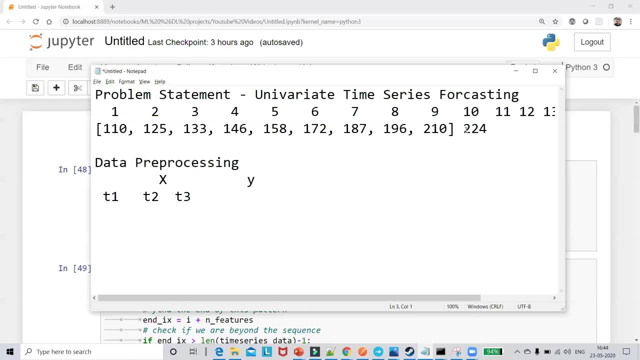 values, or nine days value. okay, how we have to divide this, suppose i let me consider one, one, ten, one, twenty five, one thirty three, you know, as my first independent features. so i have one, one zero, one twenty five, one thirty three. okay, so this is my first record. okay, now if i consider my output, 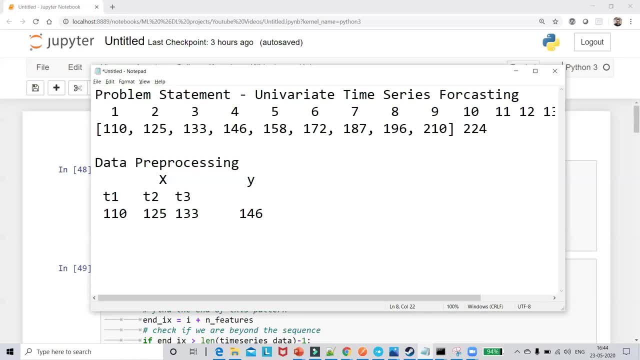 y, this should be my fourth day output. okay, so this is basically my first record. remember, guys, this is my first record. if i just select this and press a tab, oops, okay, so shift. let me just select this whole and press shift tab. so this is my first record. okay, this is my first record where my 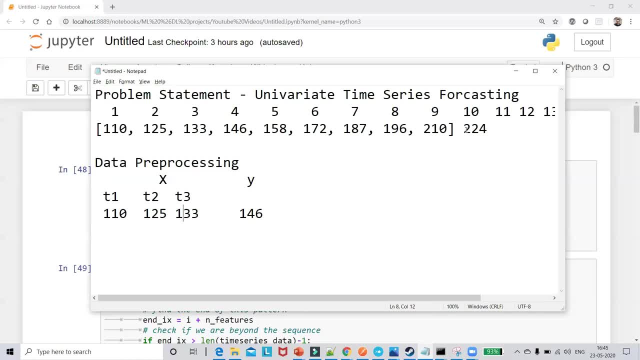 first record, independent features, are one, one ten, one twenty five, one twenty three. that basically means on my fourth day. this is my output. so this is how i'm going to prepare my output now. uh, i mean the first record of the data set. now in my second record, i will now start with 125 because, understand, i need to now. 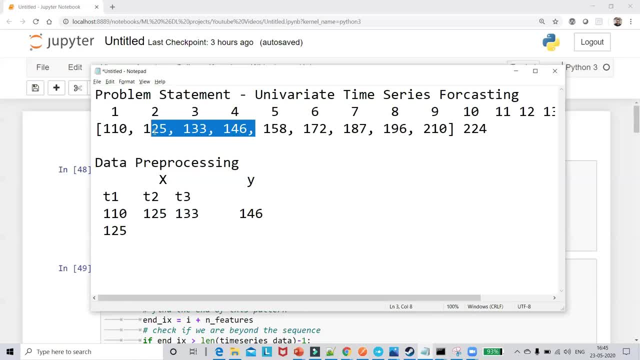 predict 158 right, and for this i have to use this past three days data right. so i have 125, 133 146 and then finally, my output will actually be 158 right. similarly what i'll do, i'll just go next step now. it will become something like 133 146. 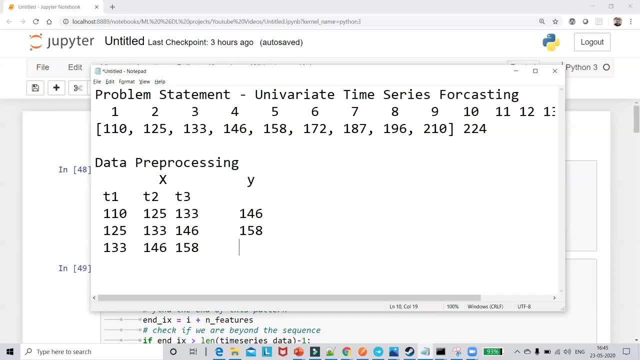 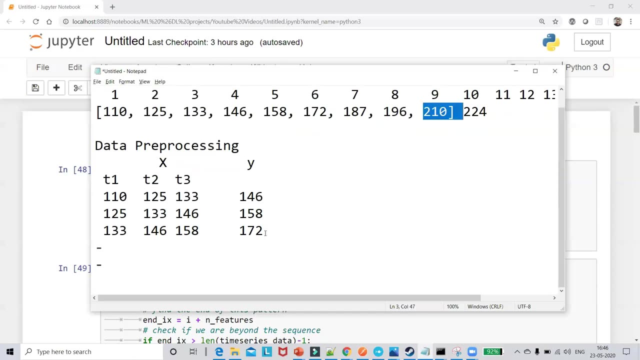 158 and, finally, my output will actually be 173. so, like this, we will continue making all the data okay. so, similarly, if i just go like this and i i go on doing this, you know. so my last record, you understand that my last output is 210, right? so, considering this, my 210 output will be looking: 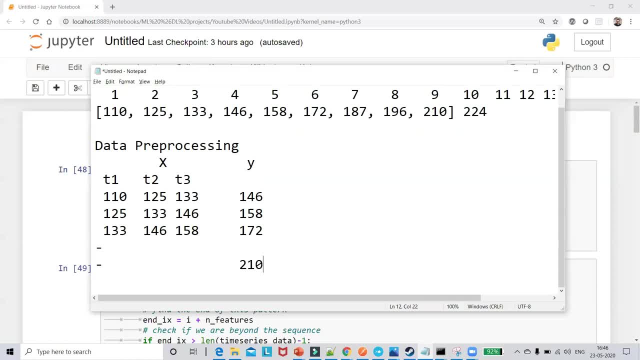 like this. so suppose this is my 210, okay, and if i see, this is my value as 196.. this is my value as 187 and this is my value as 172. so i have all these particular values, guys, and this is will be my last record, but still i have to compute the 10th day for the tenth day, my 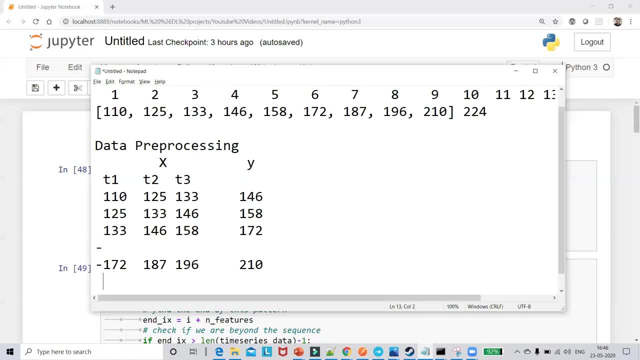 input for the data will be right, for the data will be 187, 196 and 210. right now, this value I don't have it right. so this is how we are going to do the data pre-processing. so how many number of days we have, and trust me, guys, for every. 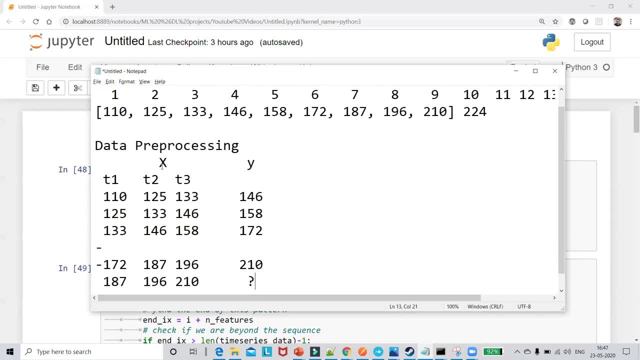 time series problem. we have to make or we have to pre-process our data in such a way that we'll be able to create our X and Y value, that is, our independent and dependent features, based on the number of time steps that you have taken. so they have taken over three times. so that told that based on previous three dates. 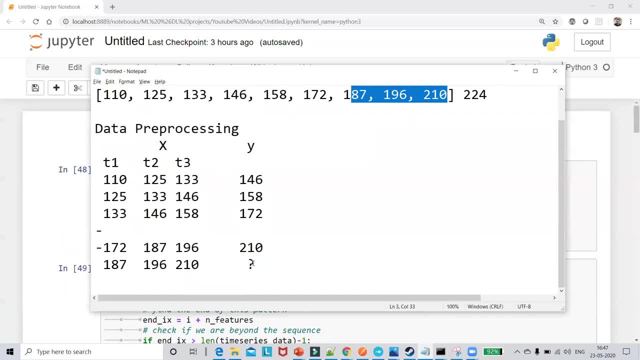 I have to actually calculate now. similarly, once I get this value for the 10 day, that what I'm going to do. I'm going to take this 3 as my independent features. then I'm going to compute for the 11th day and I'm going to do it. 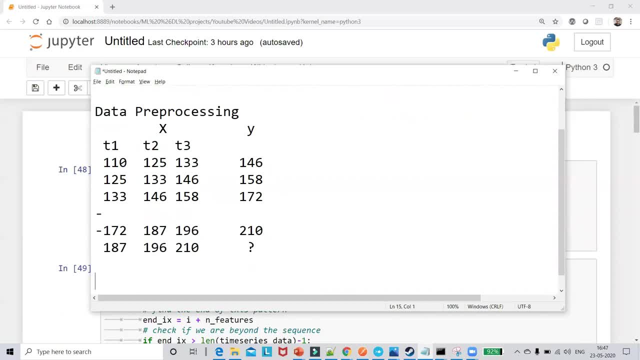 similarly, in that particular, after doing data pre-processing guys, I'm going to apply my LSTM model, a simple LSTM model, simple LSTM, RNN model, because, understand, these all are sequences, data, so RNN will pretty definitely help, right? so, after calculating, after doing that, then I'll be 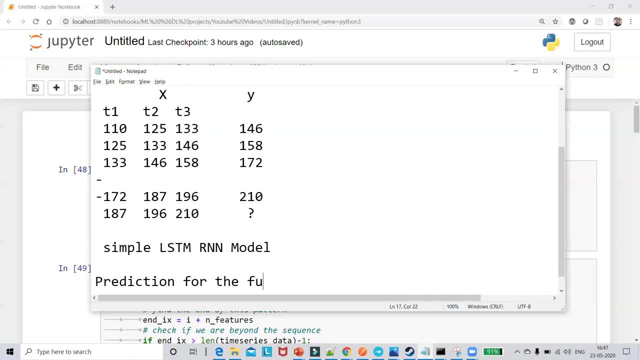 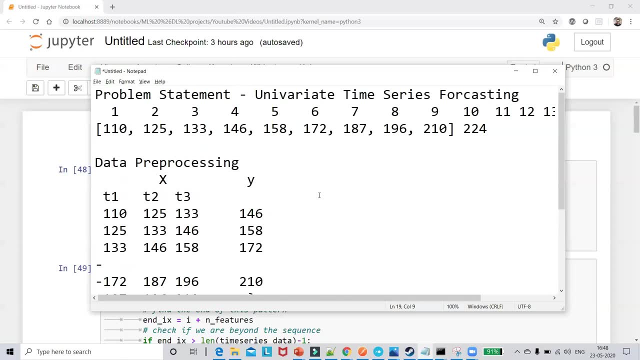 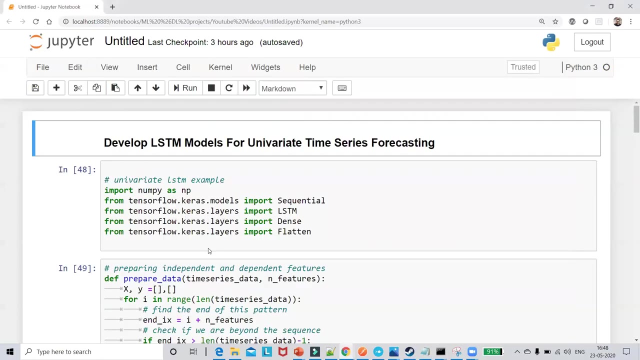 predicting for the future, for the future 10 days, and finally, we will be plotting this. so these are the steps that I'm going to show you in this particular video, what all we are doing, and we'll go one by one, okay, so let's go in now. first of all, this is the code. the code is actually given the github every. 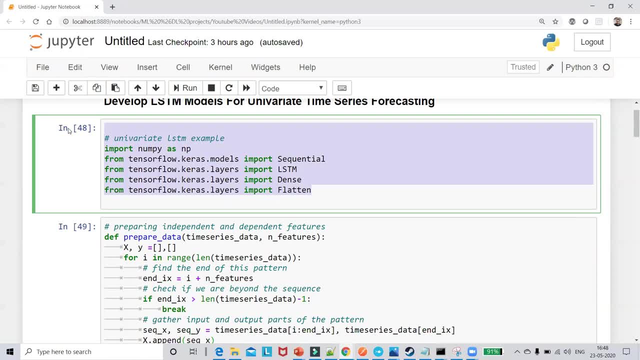 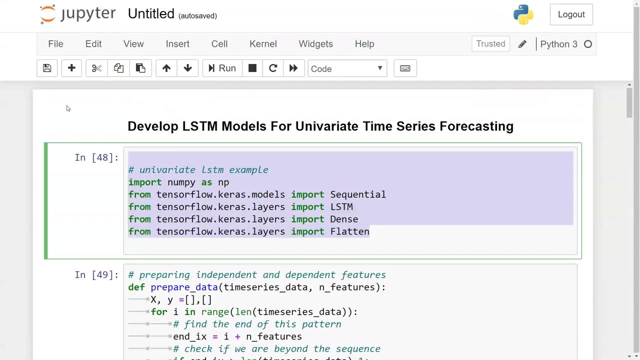 information is over there itself. now what we have to do is that let me just expand this and make it little bit zoomed in so that you'll be able to see it properly. okay, perfect now. the first thing that I'm going to do is that I'm going to import some of the 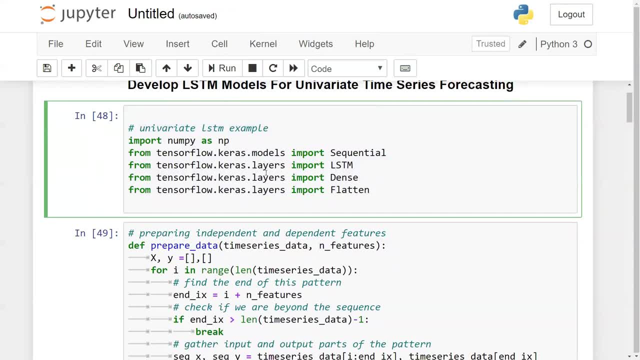 library and remember that this I'm working currently in TensorFlow 2.0. if you're not working in TensorFlow 2.0, you can remove this tensorflow, but the whole implementation is in keras in order to iterate in 2.0 or the keras integrated within the tensions fluids. right, so let's go ahead and try to see. 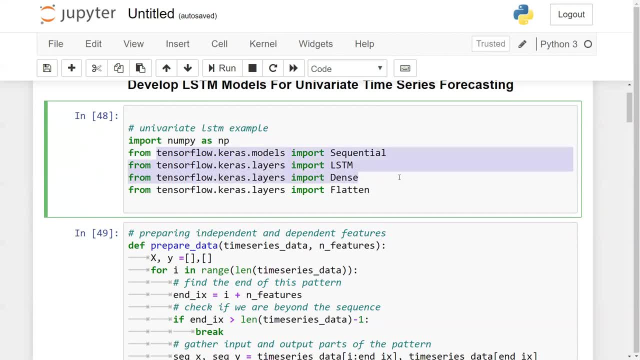 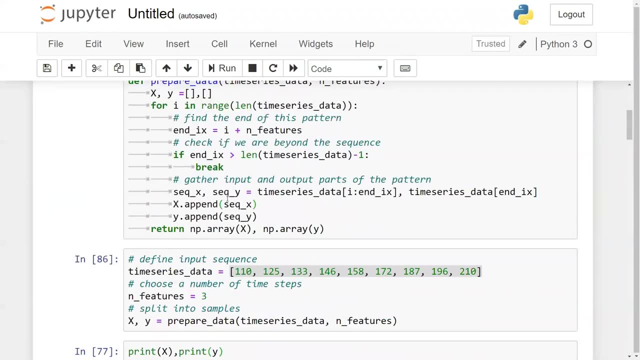 this. so, first of all, I'm going to import all the libraries that are required, like sequential LSTM, then said flattened, I'm also going to importing on fire now, and So let's go ahead with my data. So I have my time series data, which is same values that I've 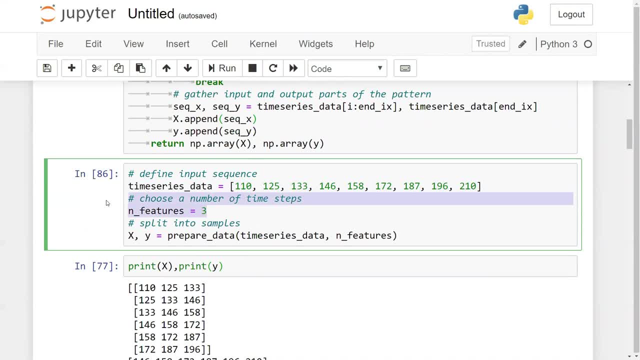 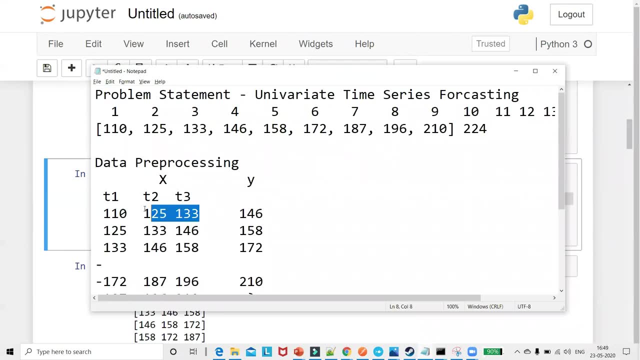 actually shown you over there. Okay, I'm going to choose the number of timestamps. number of timestamps: basically that. I told you this is my timestamps. I told you, based on the timestamps, I have to pre-process my data, right? So here again, I've taken three and you can select your. 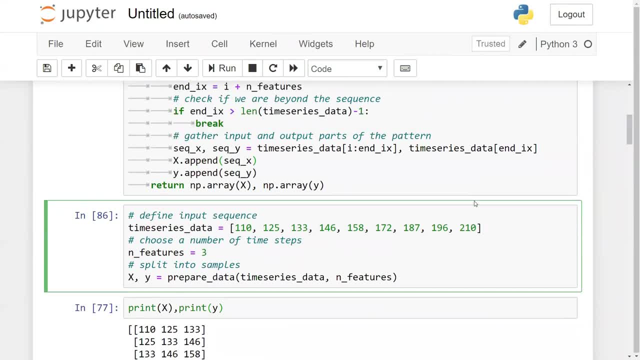 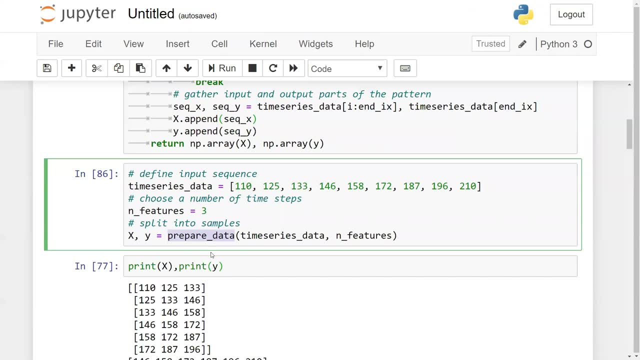 own value. You can select four, five, six, any number of values that you want. Okay, Then you can see that I'm preparing my independent and dependent features from this particular function. Now, in function, this function takes our time series data, all the time series data. 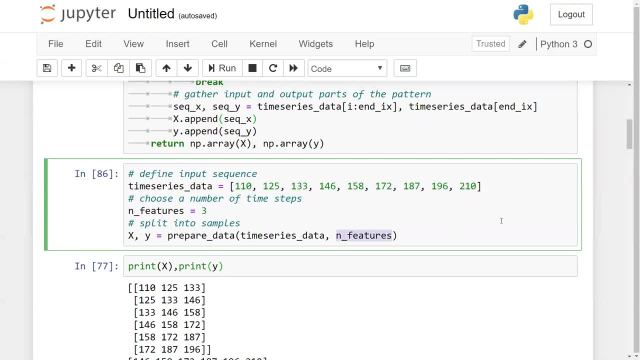 and my number of features. that is three. Okay, Now, when this is done, we'll go inside this particular function. So this is my function over here. I have my time series data, I have my number of features. So you can see number of features. So here I'm going to initialize X and Y, which 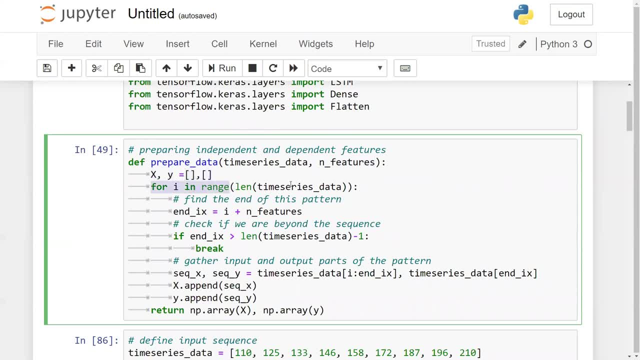 will be in the form of list. Then I'm saying: for I in range length of time series data. So I'm just going to see, I'm going to iterate through all the elements In the time series data And then I'm going to say that, for the first time, based on the number, 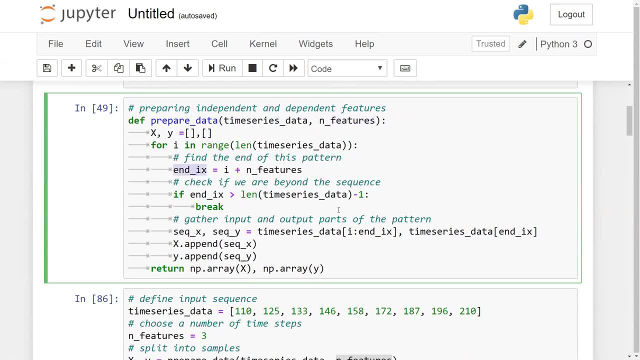 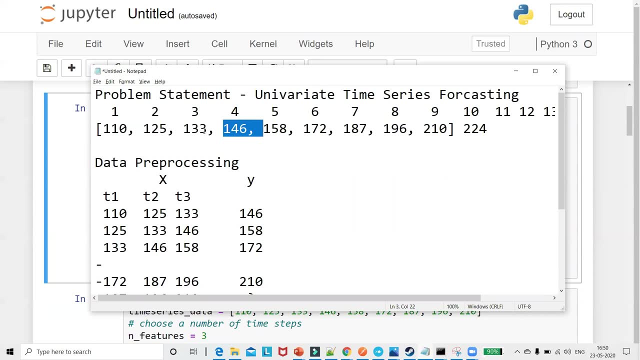 of features, just try to find out the end point and end value. Okay, Now suppose, in this particular case, when I'm iterating through this right, So my end value will be something like this right. So what I'll do, I will be you taking all this particular value in X axis and this particular 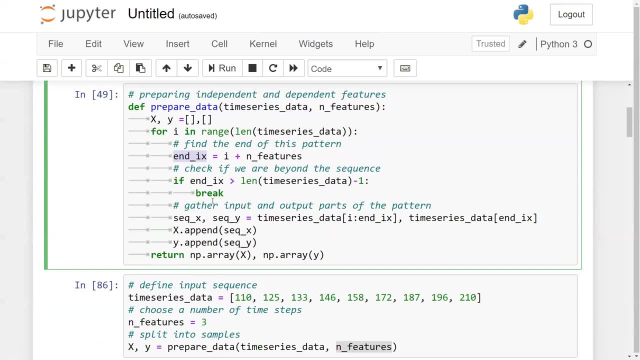 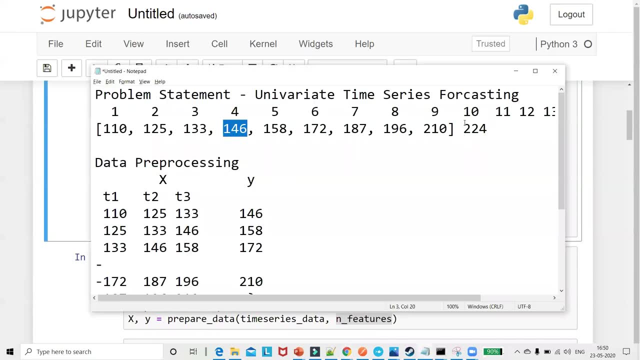 value. I'll be taking in my Y, So that is what I'm doing over here. So you can see that I'm checking whether end value is greater than length of time series data minus one. If it is greater, that basically means it has reached the end of this list. I'll come out by the break statement. 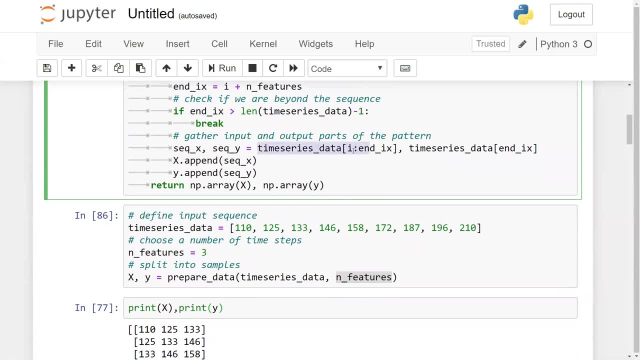 Otherwise what I'll do. I told you that from time series, data from I is equal to end of X, So that basically means from this particular value till here. I'll be taking that and I'll be storing it in my sequence: X value. Similarly, from time series only for the end underscore I: X End. 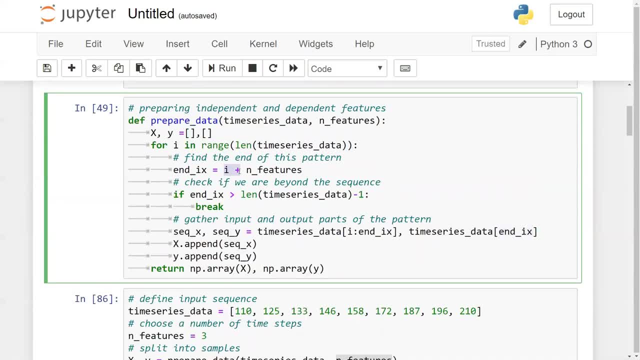 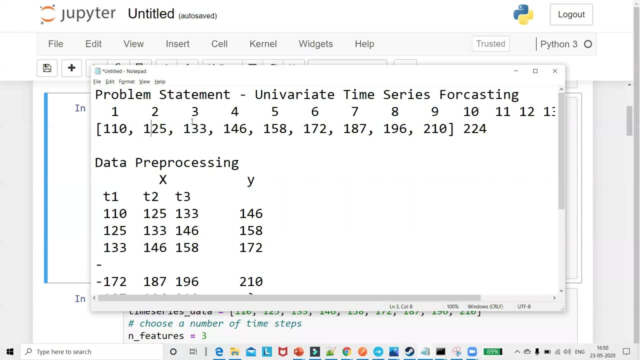 underscore I. X basically means that for the first iteration this will be zero plus number of features is nothing but three right. So third index. you can say So which is the third index? Zero, one, two, three, right. So this is the index. This will get stored in the Y axis for the first. 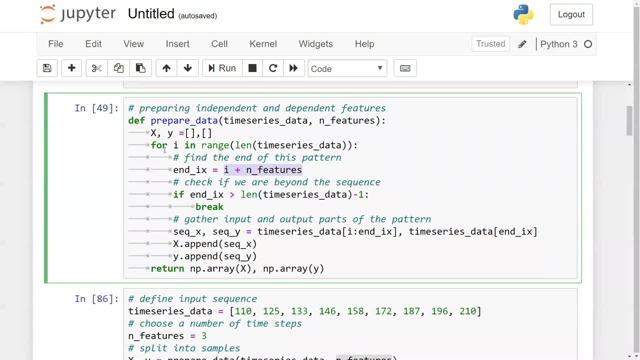 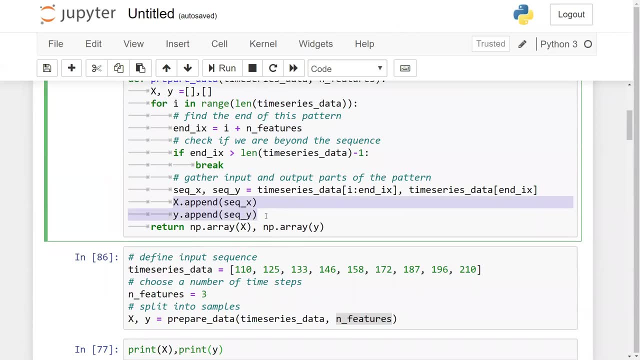 time. Okay, So that is once done, And similarly, this will be happening for all the data inside this time series. And finally, you'll be able to see that I'm appending that in my X and Y value And then I'm returning this array of X and Y. Just try to execute by your own guys, You will. 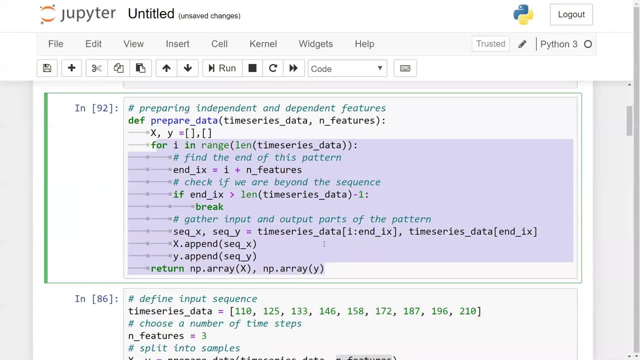 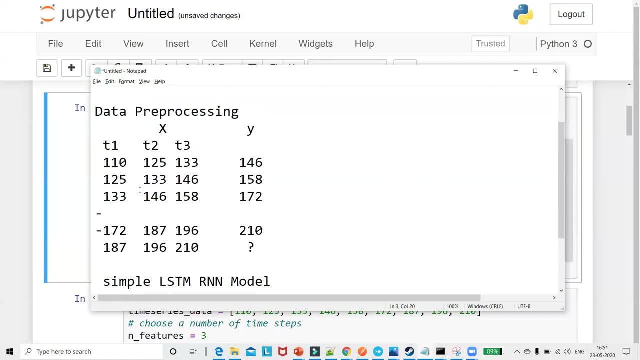 definitely be able to understand this. This is pretty much simple because you are. if you understood this logic, the code is pretty much Simple. So I've explained you in this particular manner how we are actually doing the data pre-processing. Now I'll execute this quickly. So, after executing, let me print X and Y. So this: 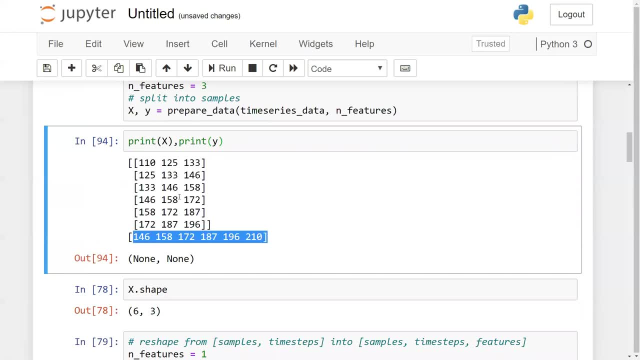 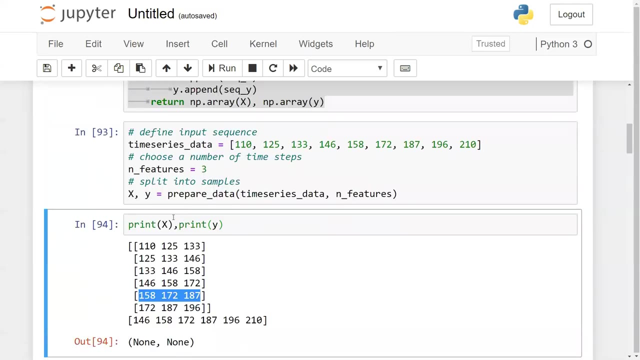 is my X values. Okay, This is my Y values. This basically means that for this X, this is my output. Y for this value, this record, this is my output for this record. This is my output for this record. This is my output. Similarly, I'm doing all these things. Now let us see that. what is the X dot? 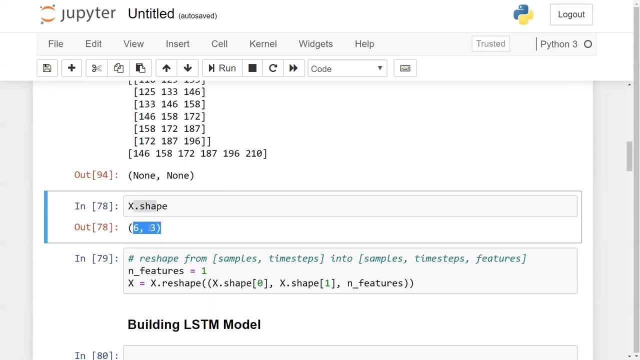 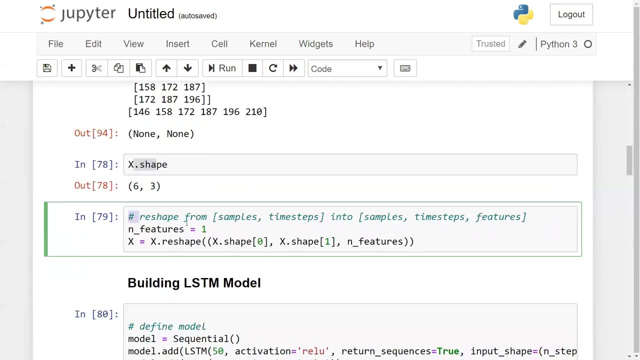 shape. X dot shape is nothing but six comma three. Obviously, it should be six comma three, because I have three features and six records. Six records has been created Now. this is a pretty important step. guys. Understand from this too when I see X dot shape: right, This is nothing. 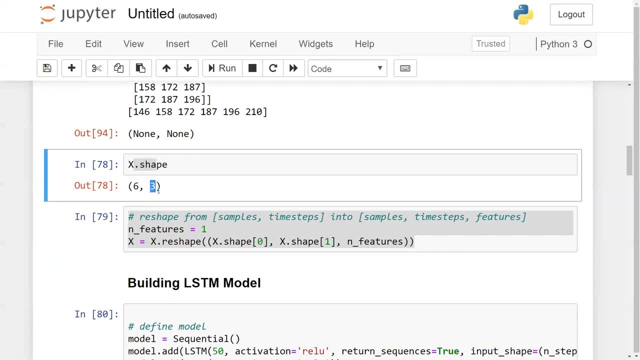 but the number of records. This is basically the number of timestamps. So timestamps is pretty much important over here. Okay, And always remember, whenever you are implementing LSTM, you always have to reshape the data, Reshape your data into a three dimensions: How, what all three dimensions are required. 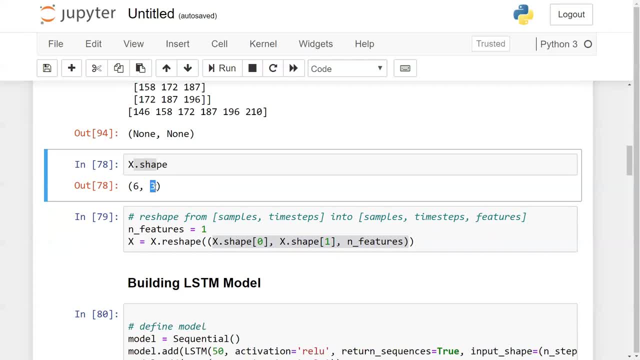 One is the number of records. The second one was with the shape of this particular, like how many number of timestamps are there, And one should be something like N underscore features. Okay, So N underscore features don't get confused by this timestamp and this. 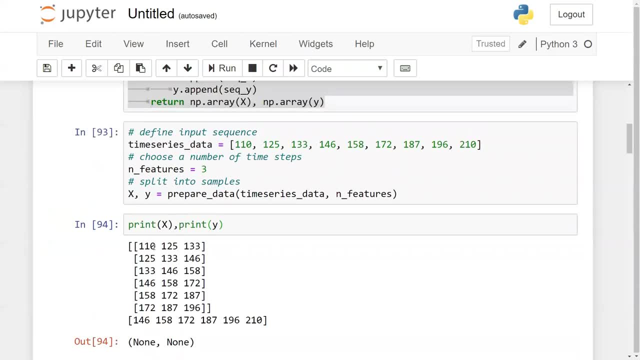 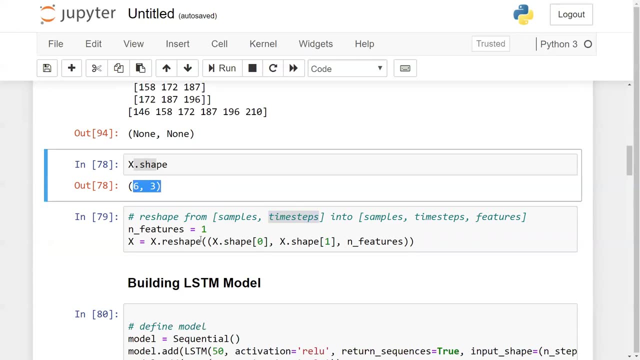 features guys. Okay, Timestamps I'm considering just like a features over here, but this feature is just something different, where we are just trying to convert this shape Into a three-dimensional shape. I feel if you want to convert this, we just have to use one over. 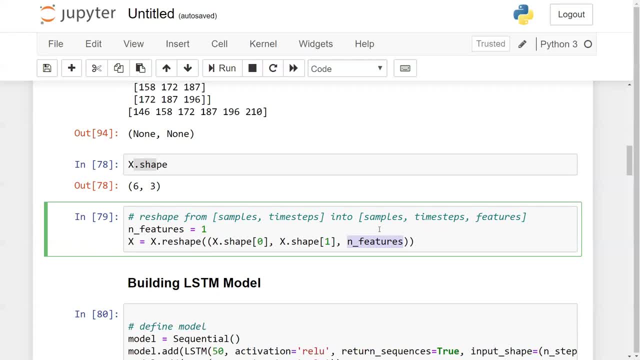 here, so that it becomes six cross three cross one. Okay, The same number of elements has been just been converted from a two-dimensional into a three-dimensional. Okay, So that is what this step is done, And this is pretty much important. You can see over here reshape from sample underscore. 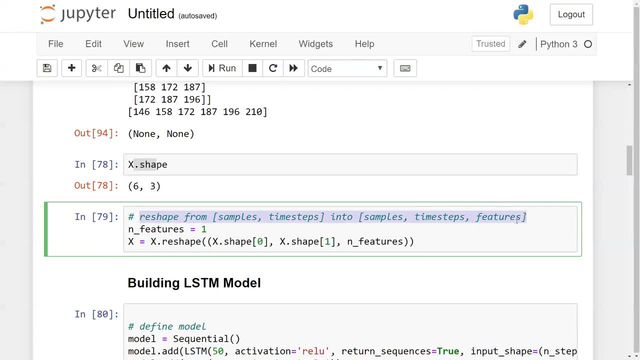 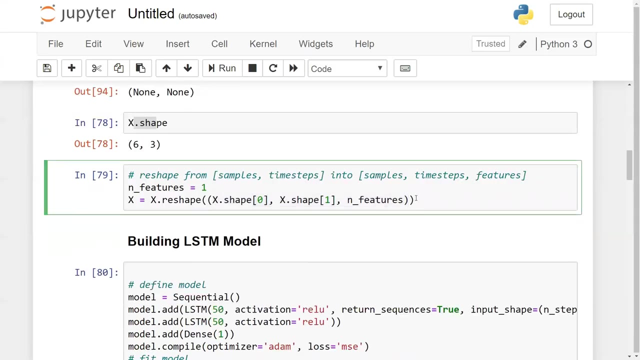 timestamps into sample underscore timestamp underscore features. Okay, So just like, this kind of example is given over here for you. but just understand, this reshape is pretty much important. Okay, We are just trying to convert this two dimension to a three dimension so that we will be able to give this as an input to our LST. Okay, And this is pretty. 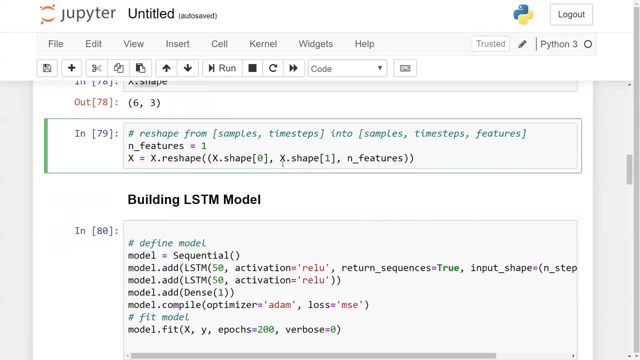 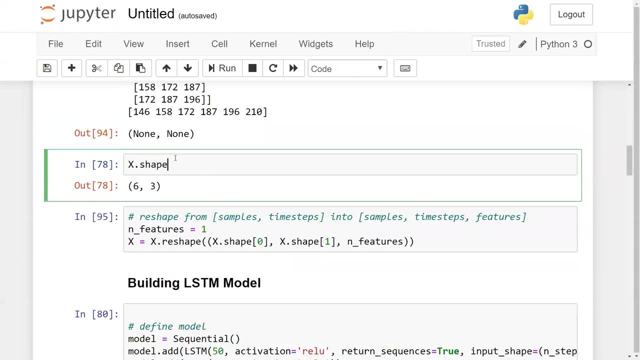 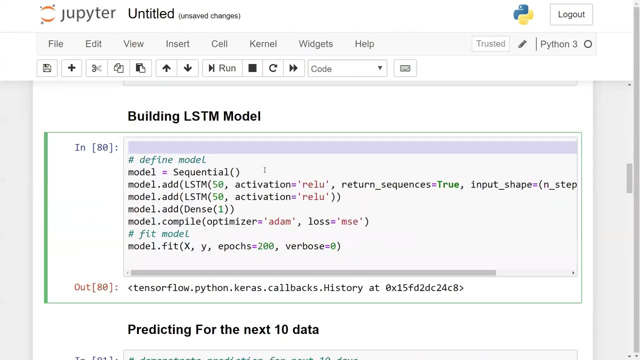 much important. Now the next step after we do this. if I execute this one, guys, you will be able to see that. Okay, Let me just see the shape. Now you can see that X safe is six comma three comma one. Pretty much simple. Now let's go ahead and try to define or build a LSTM model. This is 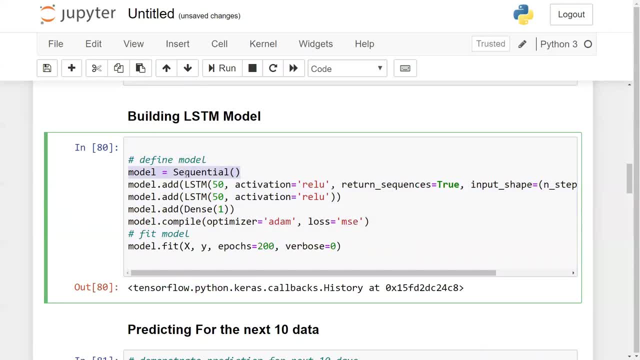 pretty much simple, guys. I hope everybody knows this. Initially I'm creating a sequential layer, Then I'm adding a LSTM layer. Activation is relu because, again I'll tell you, relu works pretty much well. with LSTM, The return sequence is equal to true. Here is the most important thing now. 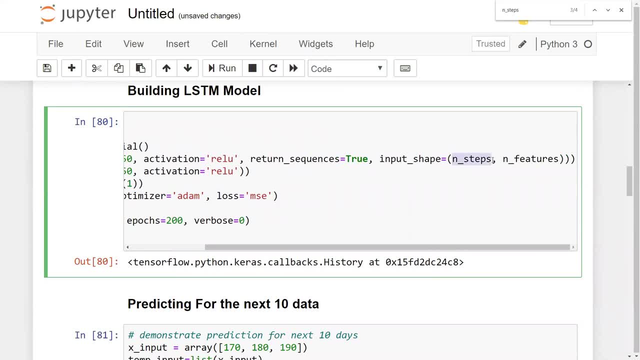 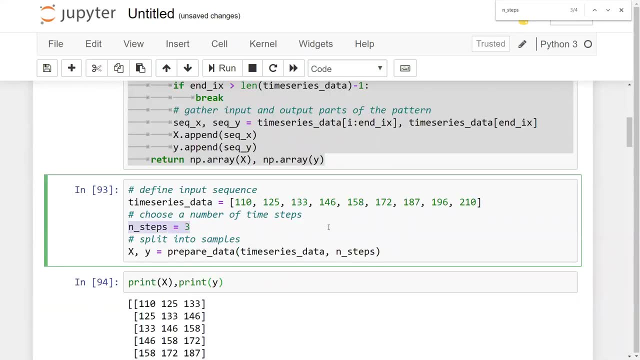 Okay, guys, this is pretty much important. in the input shape We have to give N underscore steps and N underscore feature. If I try to see what is the N underscore steps, this is basically the three value based on the number of timestamps. Or I can also say: 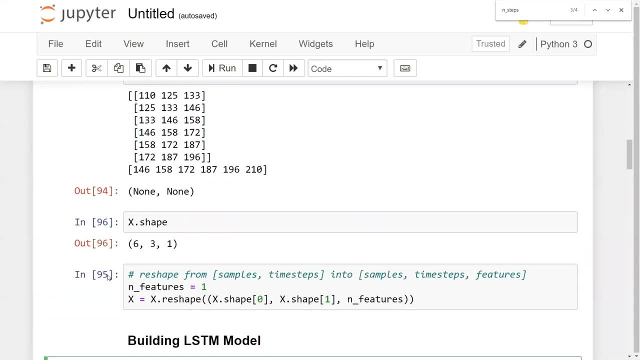 this has a number of time steps. This is basically what we have actually done with respect to the three-dimensional conversion, The last feature which we require. we have to give that as an input shape into our LSTM. Okay, Guys, in the next layer again. 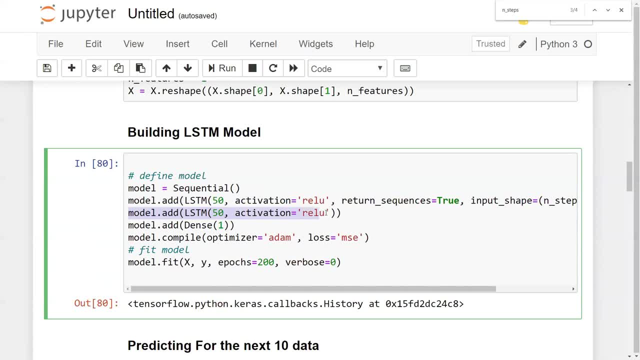 I'm adding an LSTM layer of 50 hidden neurons. Here I'm applying an activation function as relu. Finally, this is my output node, or the neural network node, basically, where I'm keeping the values one, so that we'll just need one output. Then we are doing modelcompile. 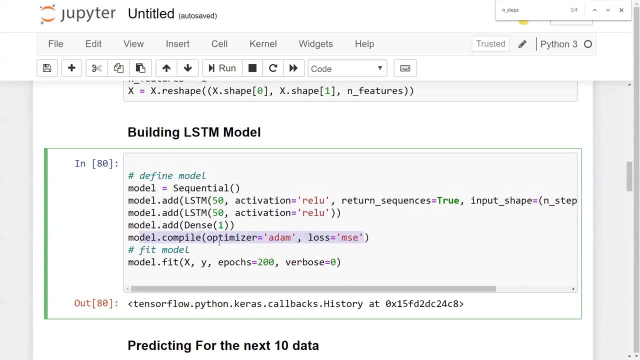 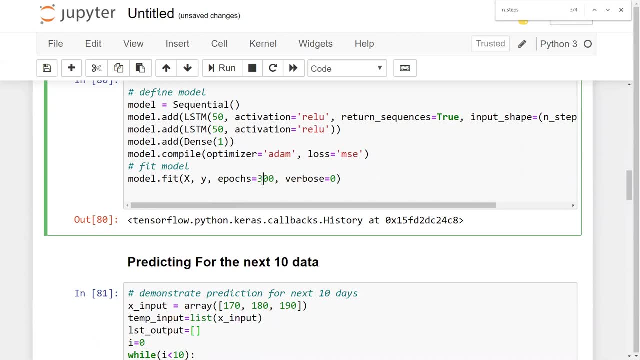 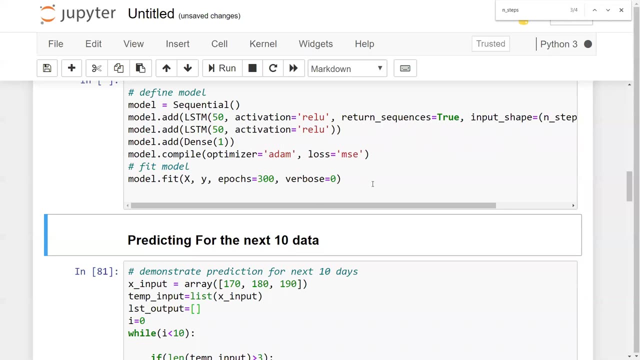 optimizer is equal to Adam and loss is equal to mean squared error. Finally, let us do it for 100 epochs and try to see. just let me increase it to 300 epochs and let me quickly fit the model over here. So we will be fitting the model. Let's see. we'll face any errors or not. 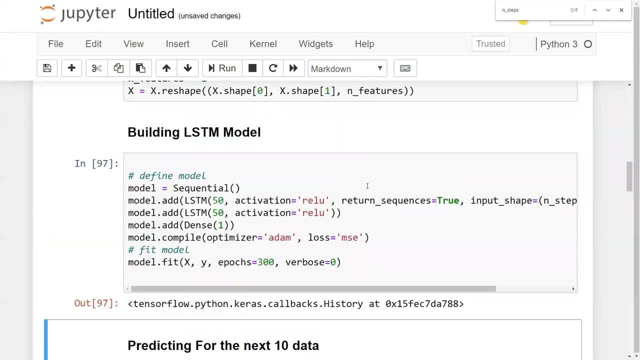 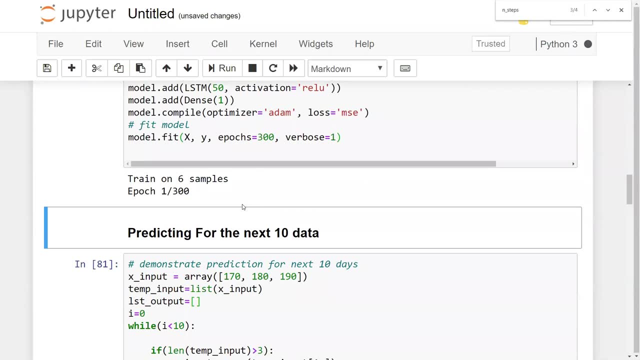 or it will just get executed quickly. Yes, it has got executed quickly. If you really want to see verbose with verbose is equal to one, you'll be able to see all the epochs, that how it is basically taking place. And here you can see all the epochs so quickly. And since the data 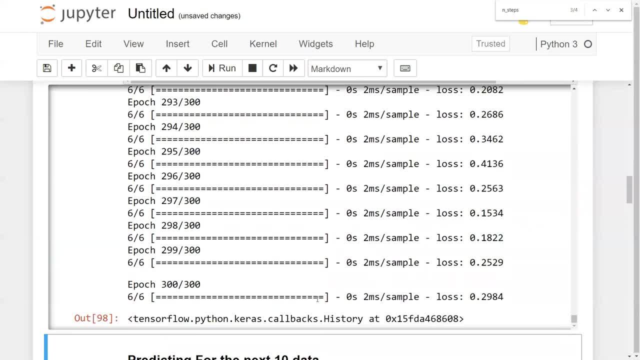 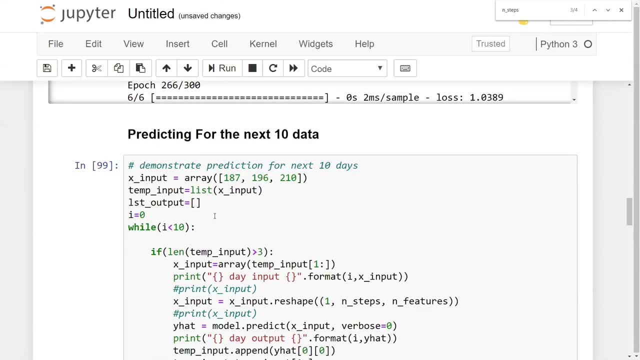 set is very, very small, guys, and you know the execution time will be very, very less. Okay, So, this, once my fit is done. okay, now, this is the most important step. Okay, guys. So the next step is that I'm going to predict for the next 10 days, after I've actually fitted my model. Now, 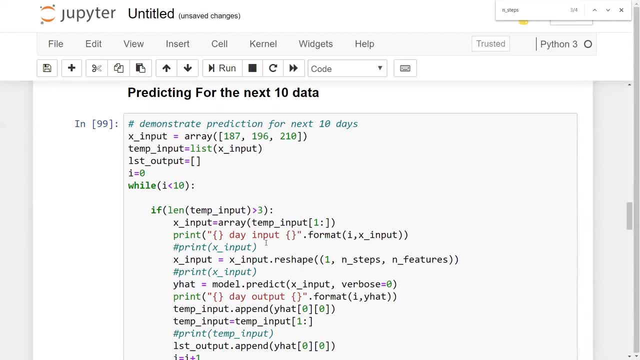 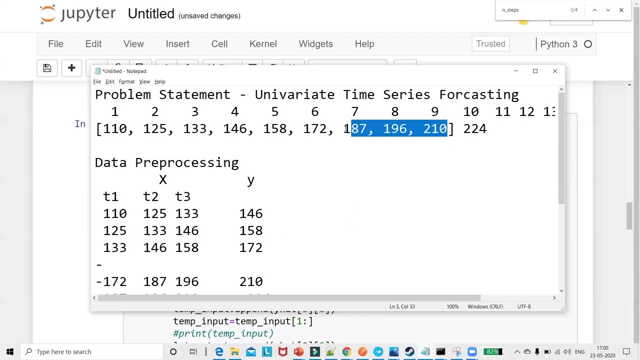 this step is pretty much important. What I'm going to do, as I've shown you my data set already for the 10 day computation, you know I will be taking the previous three days data. Okay, So previous three days data I'll be taking over here and then I will be computing the 10 day output. 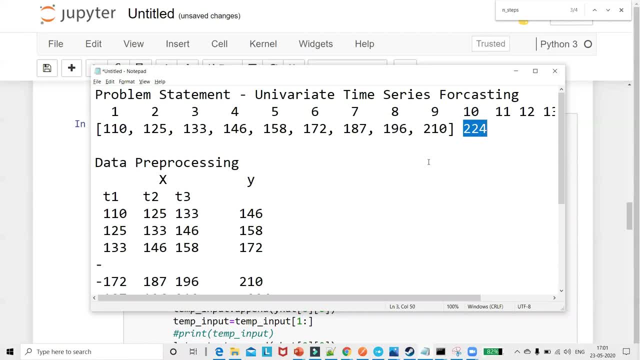 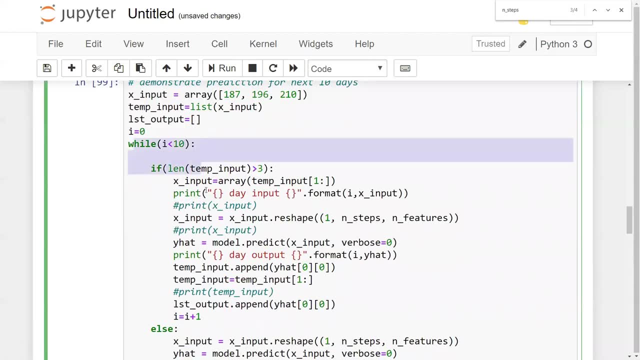 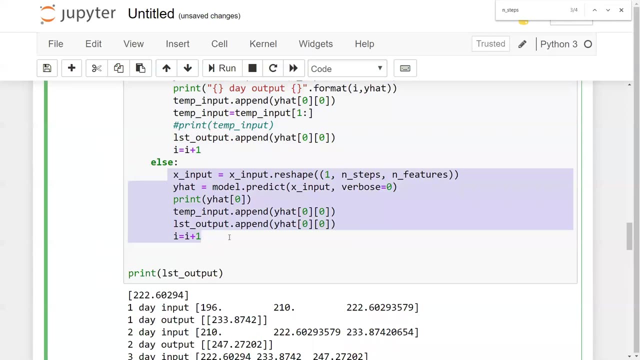 After getting the 10 day output, I will again append this to my input so that I can compute my 11 day. So for that I have written this particular logic. This will be happening for 10 days. Okay, There are two statements. If an else first loop, it will go to the else block, you know. 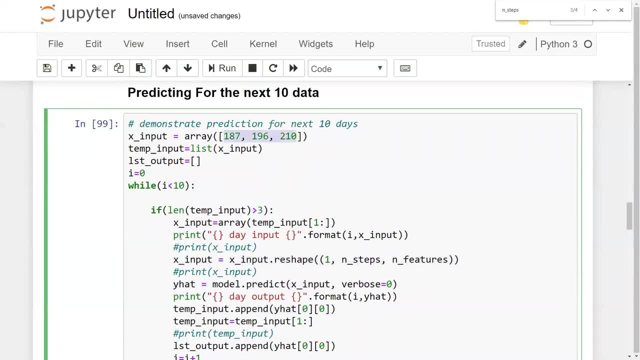 because we already have the three days input Right In this particular block. as soon as it goes, we are basically adding: suppose we are, once the output is got, we will be appending in this particular list And then we'll be taking this last three values to calculate the next. 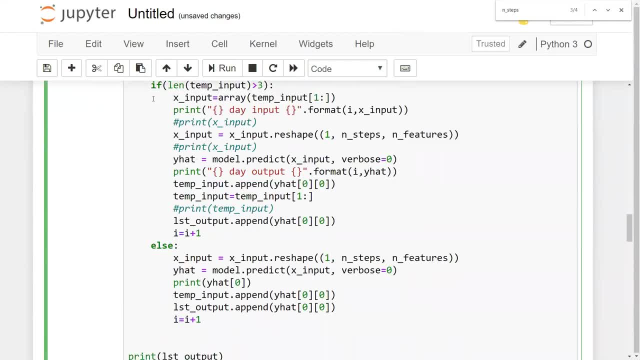 value. So similarly, we'll be going on. I would suggest just go through this logic. I have written this particular logic to get the output. Okay, So you will get the output. you will get the output here because you will be taking these 10 days. you are taking the three days input, so that now, if I am adding, 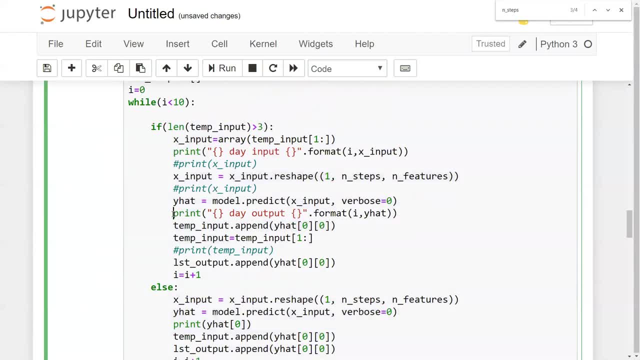 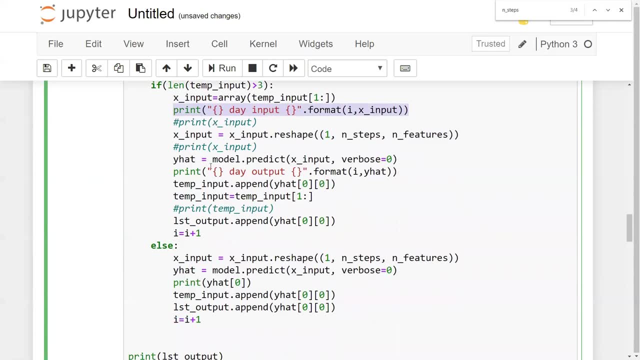 For this first three days, just keep doing. I have written this particular logic to get the output. Okay, so you will be taking the okay, so you will be also able to see that i'm printing the values also over here, like what is the first day input, what is the second day output, what is the first day output, and all like this. 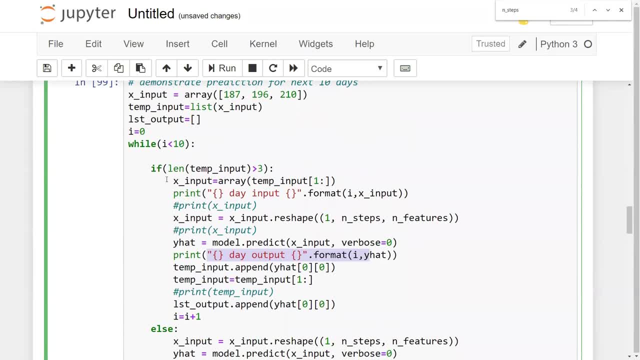 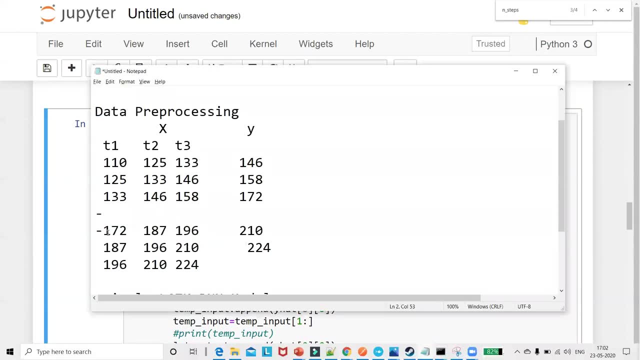 right, so i'm printing this. i would suggest, guys, this is a very interesting logic that i have written. just go through this and you'll be able to understand. but understand the logic is something like this: okay, suppose this is my ninth day output, right? i will append this over here to my input and 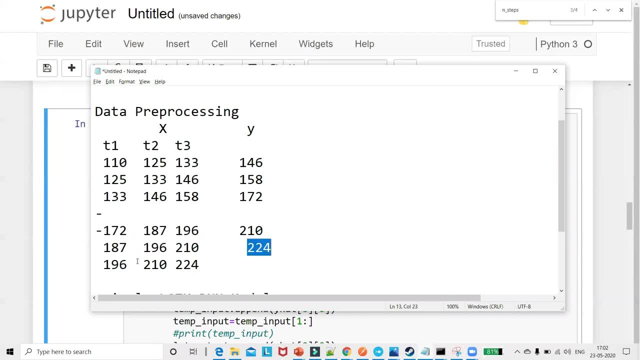 it will start from 186, like this, and then i'll compute the next day output. then again i'll be taking this particular value. this will become my input, and again i'll compute the output. then again i'll be taking this 3 as my input. so that is what this if and else logic will actually do. 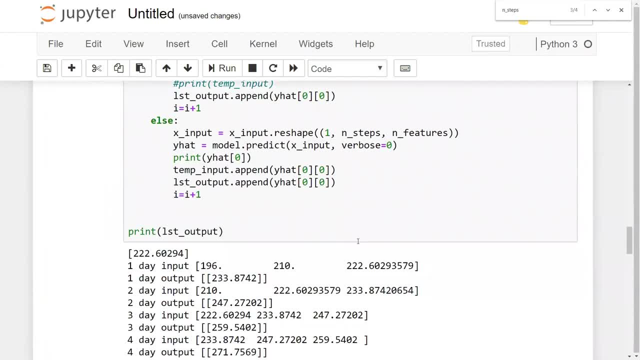 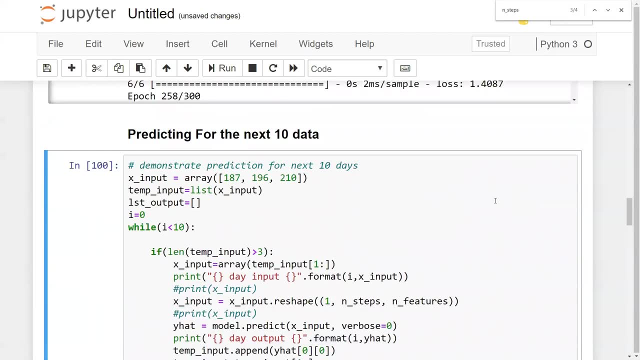 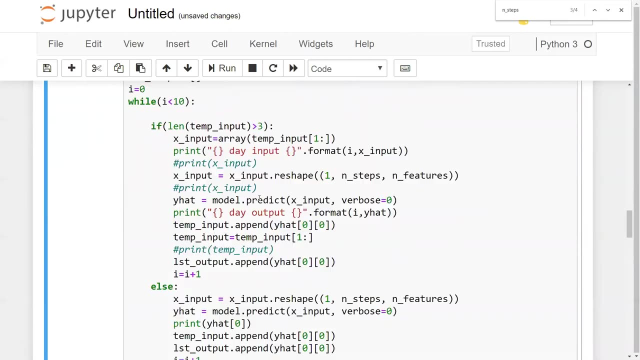 okay, so let me just execute and show it to you. so here you'll be, seeing that. okay, the first day input is 196, 210, 222, right? so this is my first day input. if you really want to see, uh, the first day input, then what i'm going to do after this is that, uh, remember, i have given this as my first. 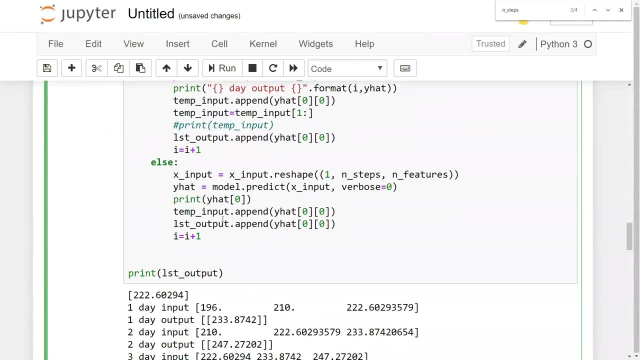 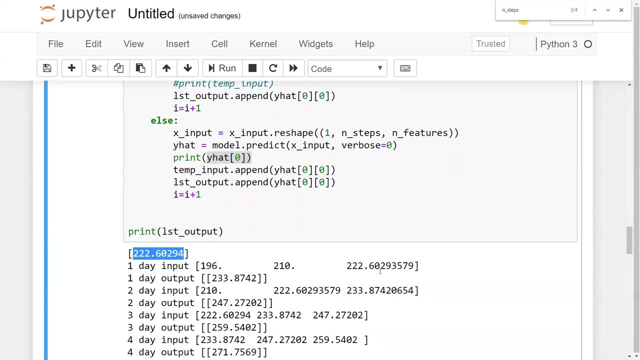 day right: 187, 187, 187, 196, 210. if i go and see in the else block, i have printed y hat of zero. so this is basically my output. first day output. now what i've done: i have appended this over here inside my list and you can. 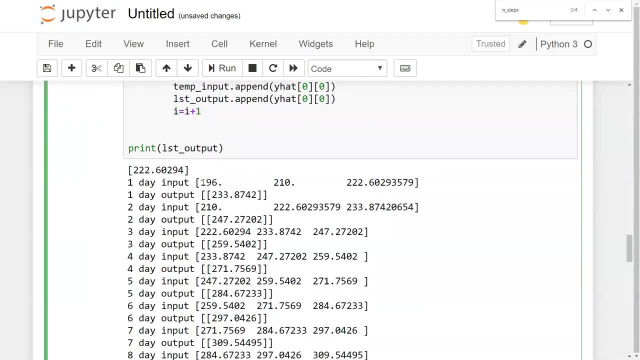 see that i skipped this 187 right, so it is starting from 196, 210, 222, then for this i will be getting this particular output. then what i'm doing again, i'm appending this to this particular list and it is starting from 210 till this particular value. again i'm getting the output as 247, again in the 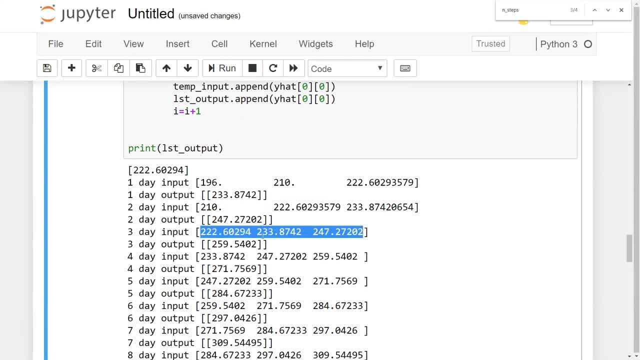 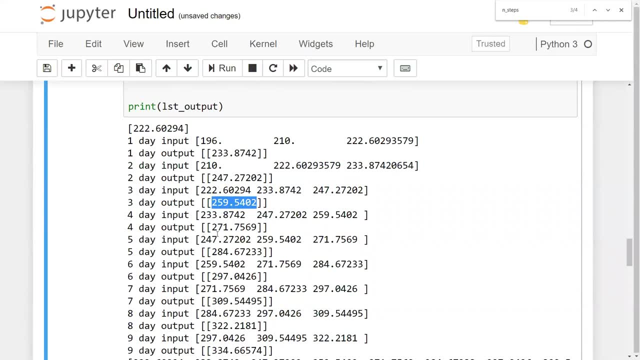 next day my input will be looking something like this: you can see that it is clearly given in front of you what are the output i'm getting for a specific day and for the next day, input that is actually added at the last, and remember always the size of this will be three timestamp, okay. 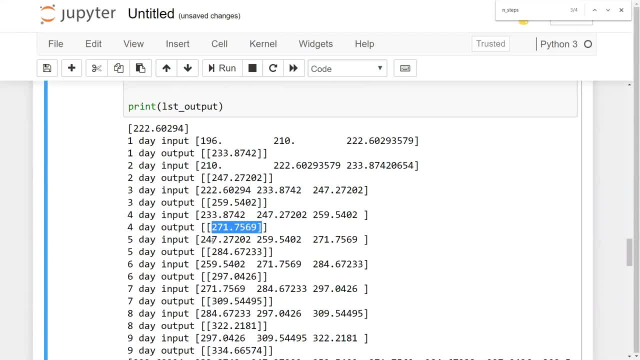 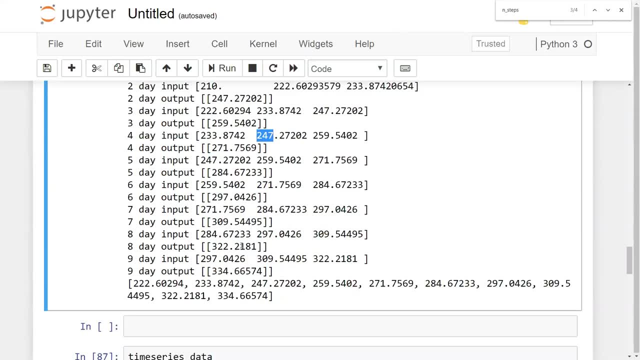 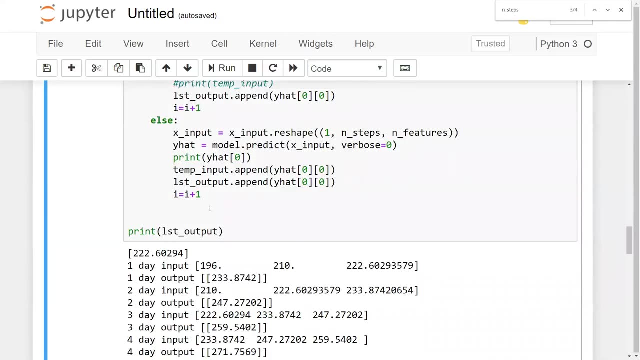 three timestamp and again we'll be getting one output. again i'm adding this to 71 over here inside this particular list, and again i'm taking it from 247. so like this it will continue. okay, this is all my final output for the next 10 days. okay, this particular list and this particular list. 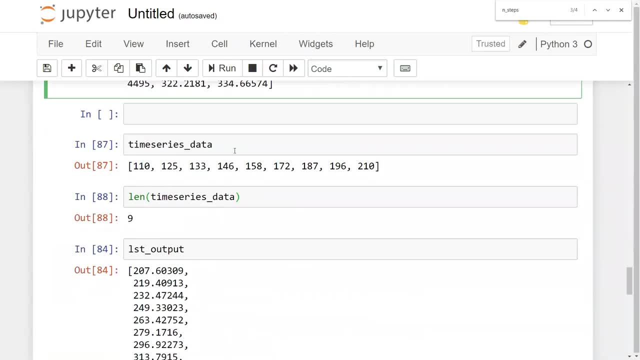 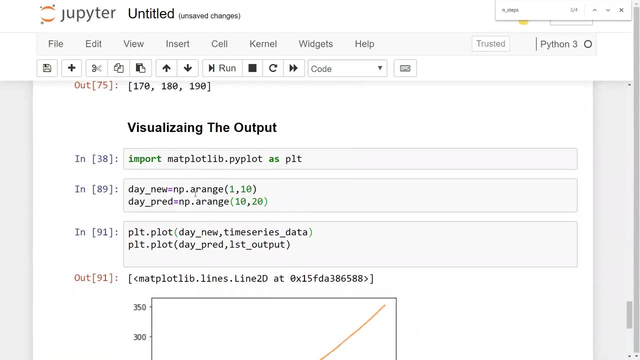 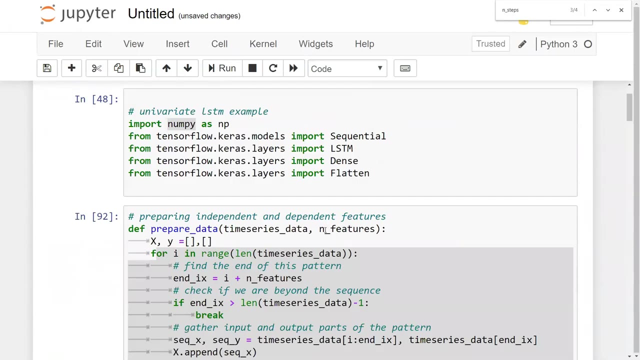 is actually stored in list underscore output. now, what i'm going to do? this is my time series data. this is the length. i'm going to create some date for this, okay, so first i'll create the date of nine days, right? so this, this data that we had, right, this, this, the whole data, uh, that, if i show, 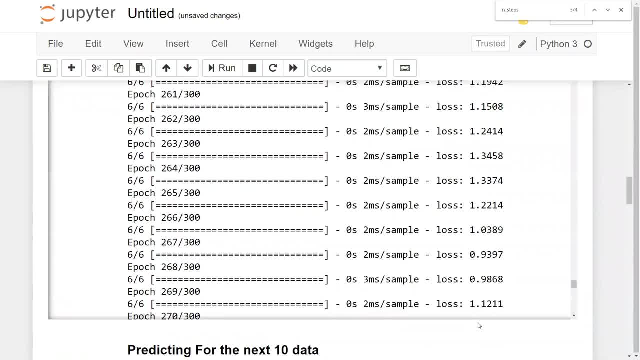 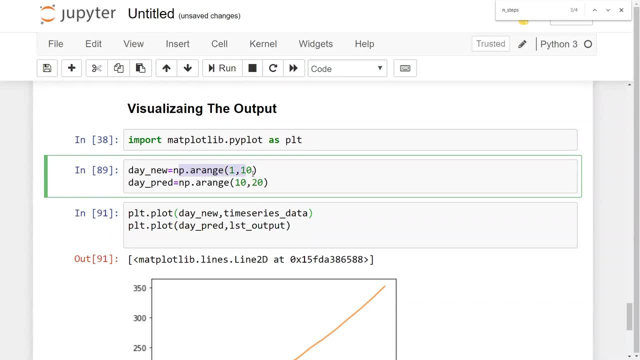 you, this whole data was for nine days, right? so i'm just going to create the date for those data, just like day one, day two, day three. so here i've just write the written np dot arrange one comma 10. then i have written: uh, the prediction data is from 10th to 28th day, right, so two days. 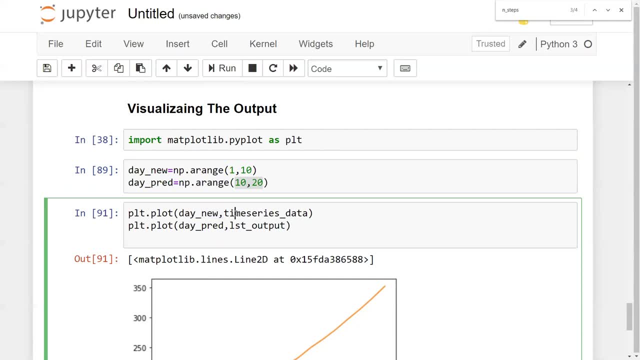 pattern i have written. i have just plotted day comma new with time series data- this was my data set that i had- and day underscore pred, which is basically my predicted data set from 10 to 20, and i'm plotting it with my list output. now, once i execute this, you'll be seeing this amazing results. 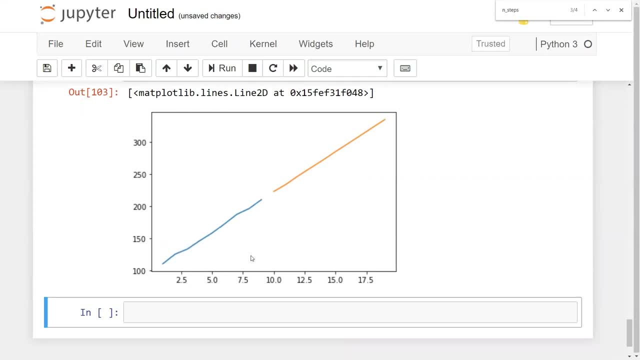 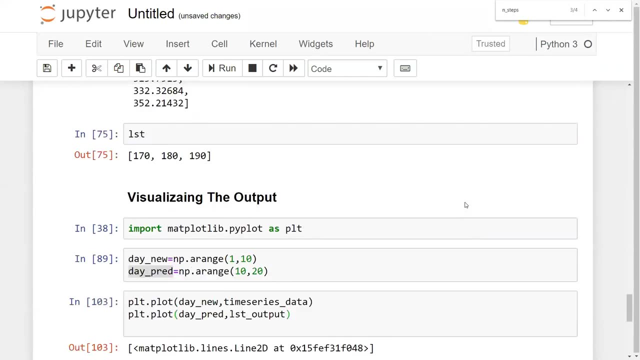 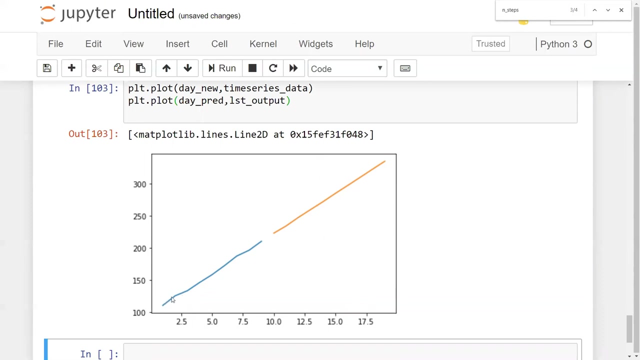 now, here you can see that this is my data, that i have, and this is the data that is being forecasted by the lsdm right, isn't it amazing? i know you will be thinking that, krish, the data will always not be like this. yes, the data is not always like this and you cannot just uh, here you can also see that. 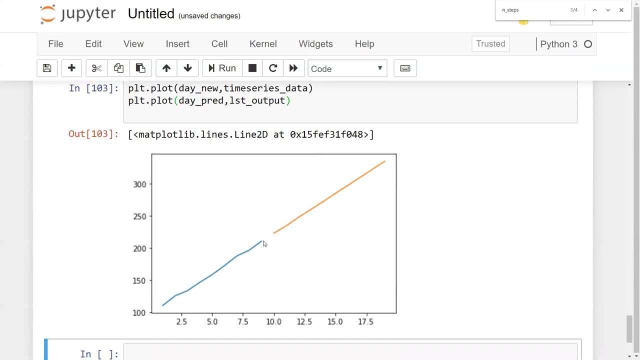 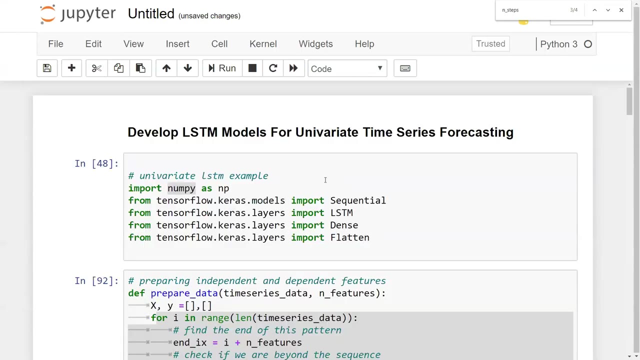 right, after some point, it is coming down, it is going up, it is coming up and going down. right, so, similarly, this is just done, some kind of predictions, which is pretty much similar to this kind of line, right? so this is how we have done this particular visual analysis. uh, sorry about the visual analysis of the time.